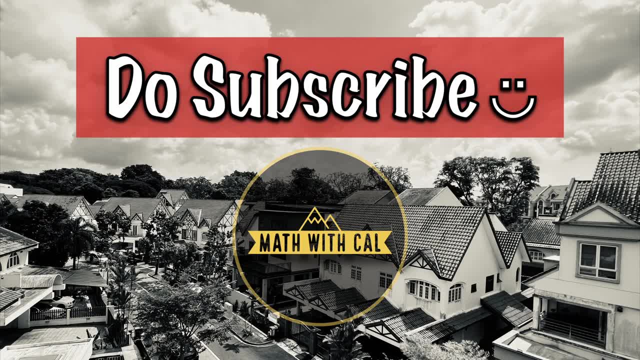 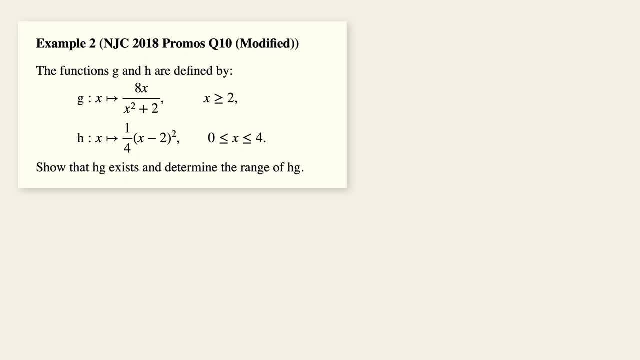 to the next example. do remember to subscribe to see more valuable math techniques. that will benefit you Alright. moving on to example 2.. Again, we need to show that the function HG exists. So for a composite function to exist, the range of G must be a subset of the domain of H. 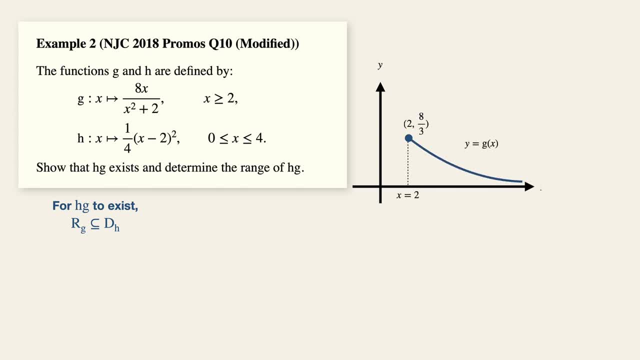 Now let's sketch the graph of G with the given domain to help us visualize better. So the range of G is simply from 0 all the way to 8 over 3 inclusive. Do note that this is a curved bracket over here, as the graph will never touch. y equals to 0. Whereas this is a square bracket to indicate: 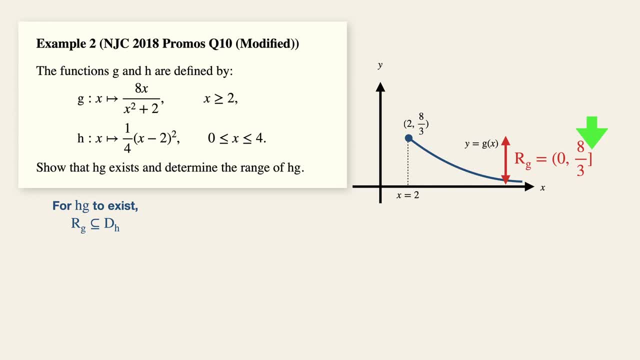 that the range is up to and including the value 8 over 3. because of this given sign over here. Now, the range of G is indeed a subset of the domain of H, So we can simply read off the domain of H given by 0 to 4.. Thus we conclude that the composite function HG exists. 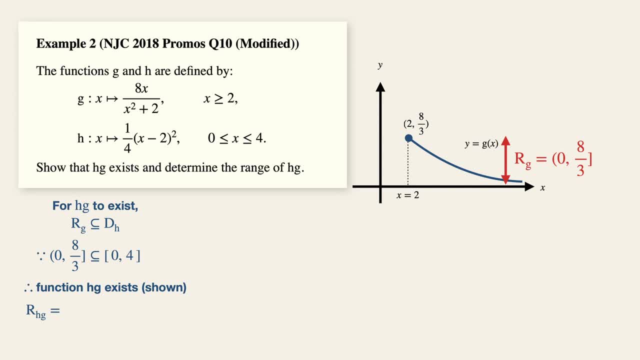 Next to find the range of HG. it's simply the range of H, But remember we need to restrict the domain of H to the range of G. Now let's make it a habit to do a quick sketch of the function H, Similar to the previous example. the range of G is now the domain of H. From this domain, 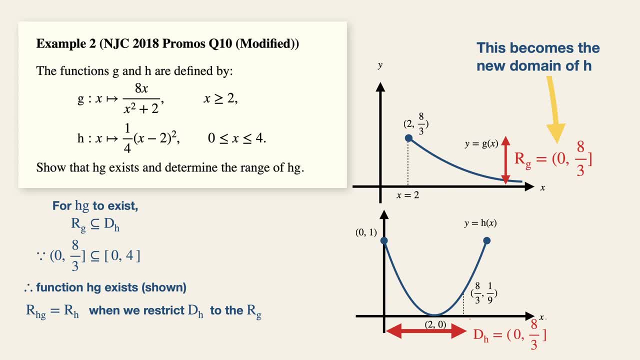 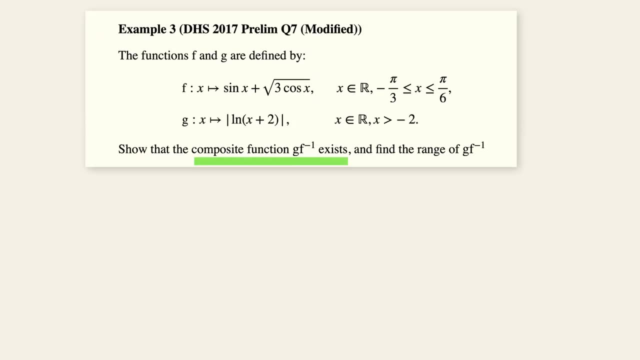 read off Or find the corresponding range of H, So it stretches from 0 to 1 inclusive. To get the value of 1, simply substitute x equals to 0 into function H. Now let's move on to the next example, where we now need to prove that the composite function GF inverse exists. So bring up the 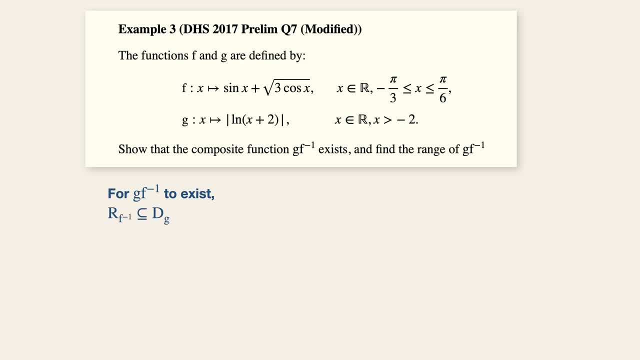 condition again For this to exist, the range of F inverse must be a subset of the domain of G. Before we do that, let's look at the next example. So let's look at the next example. Before we jump into sketching the graph of F inverse to get its range Now, do recall that the 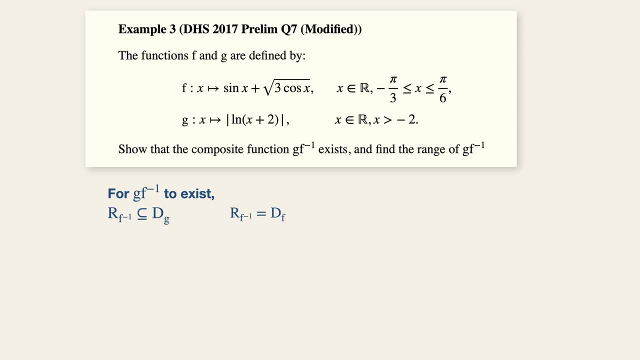 range of F inverse is equals to the domain of F. So, very quickly, the range of F inverse is from negative pi over 3 to pi over 6 inclusive, And this is a subset of the domain of G, which is minus 2 and infinity. Therefore, the function GF inverse exists.